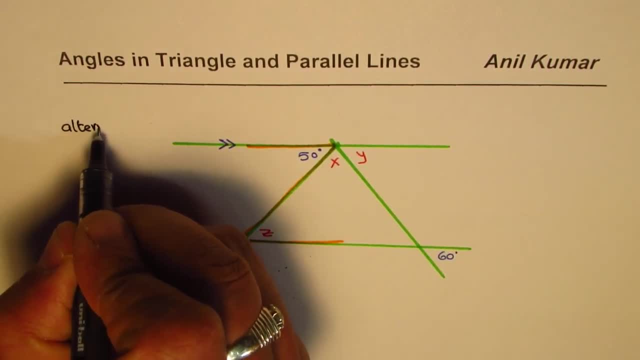 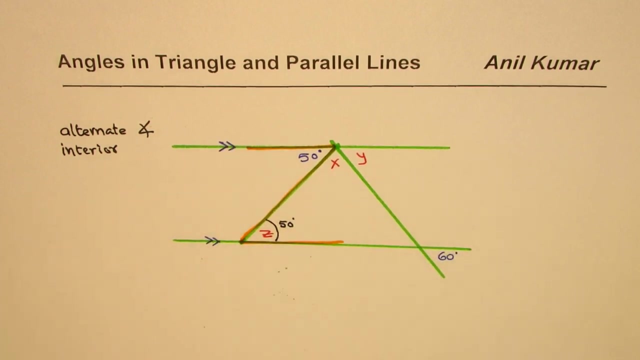 So what we get here is alternate angles, And these ones are interior alternate angles, right, They are always equal. Therefore, Z, this angle should be equal to 50 degrees, correct, That becomes 50 degrees. Now, the other angle given to us is 60 degrees. 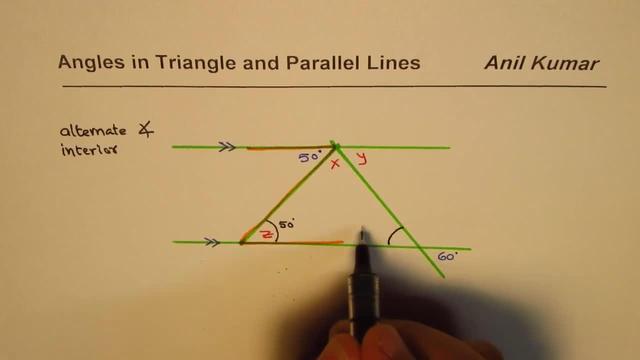 And vertically opposite angle should be 60 degrees. right, So you could do like this: Once you get that, you can find X. The other way to find X is that you can see that Y and 60 degrees given to us are corresponding angles. 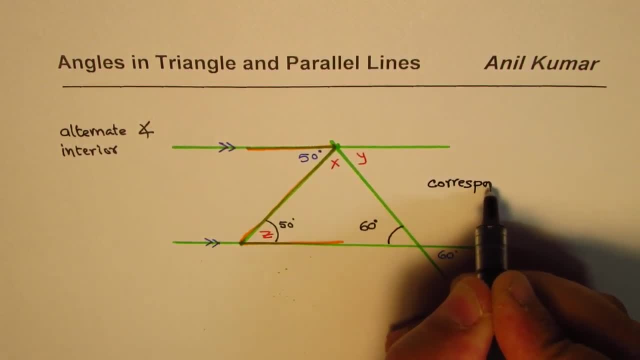 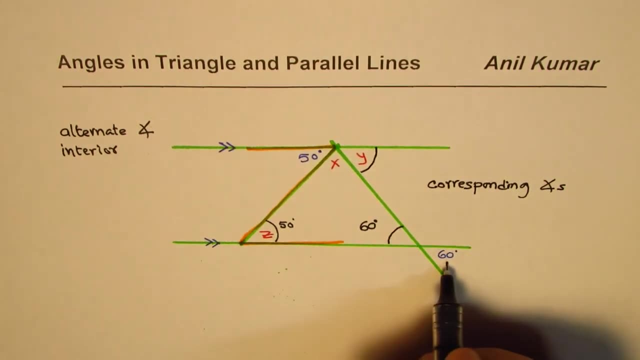 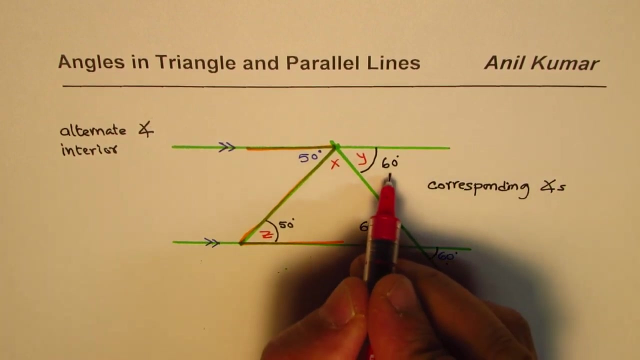 So these are called corresponding angles, and corresponding angles are always equal. So why this angle should be equal to 60 degrees, right? So because they are corresponding angles, So these ones are equal, since they are having similar position. Do you see that? 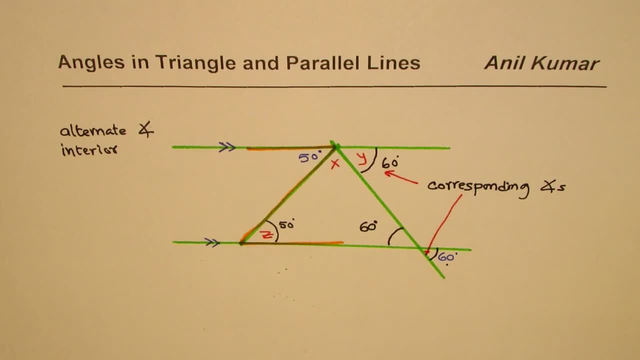 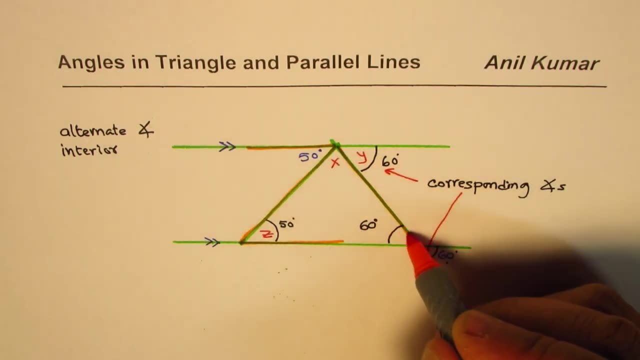 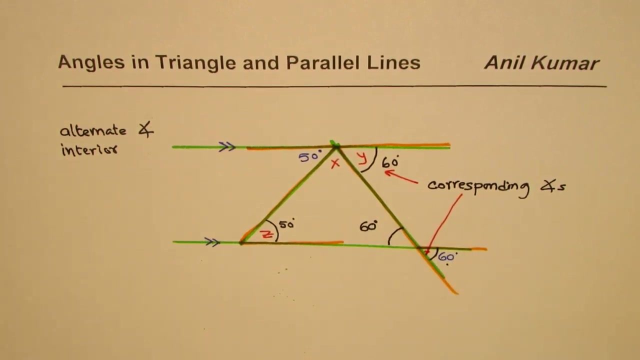 So under this line they have similar position and therefore they are equal. And the pattern they make is kind of an angle, It's kind of an F, right? So this is an F structure. You see this kind of an F. So look for these patterns to figure out equal angles, right? 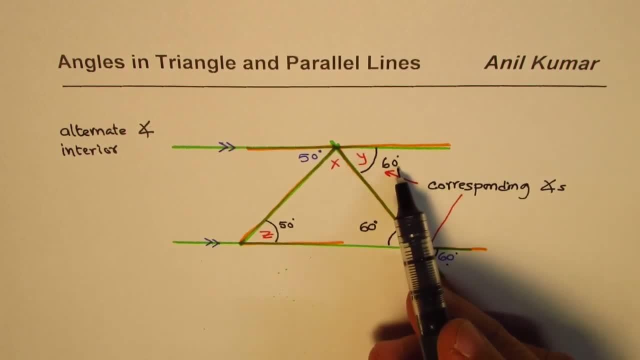 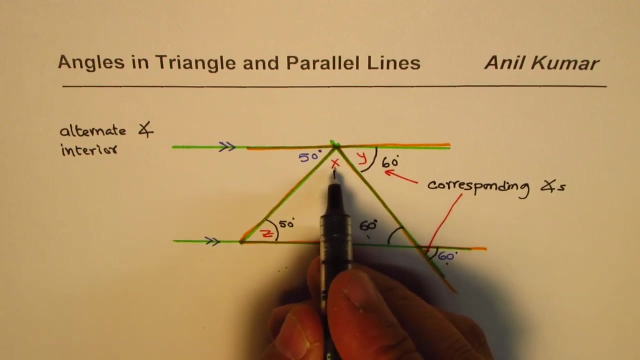 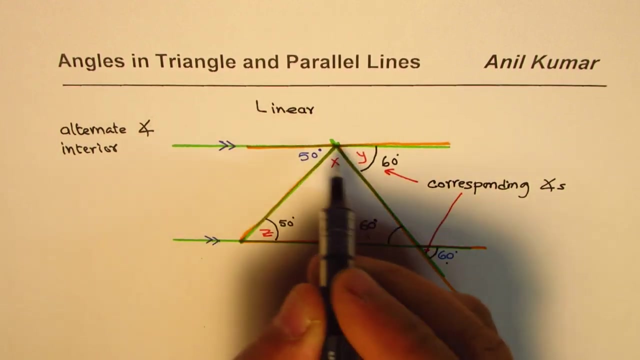 Now, once you get 60 degrees and 50 degrees on a straight line, X is 180 minus these two. So you could find X either from this calculation or from the triangle calculation correct. So the value of X should be be: let's take linear pair, so the straight line is called linear right, so linear angle. 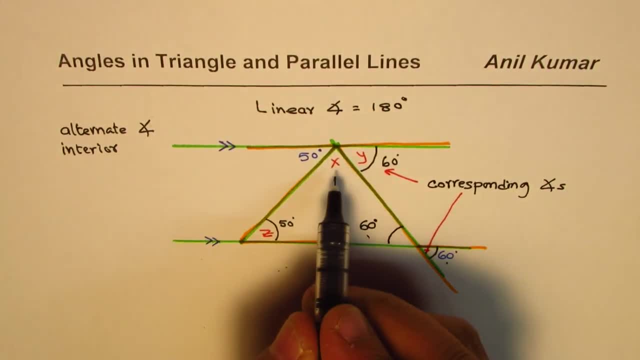 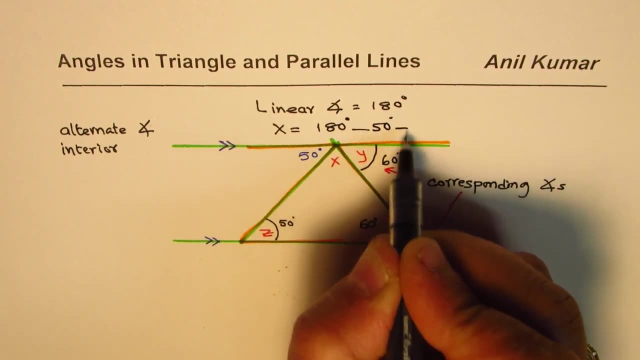 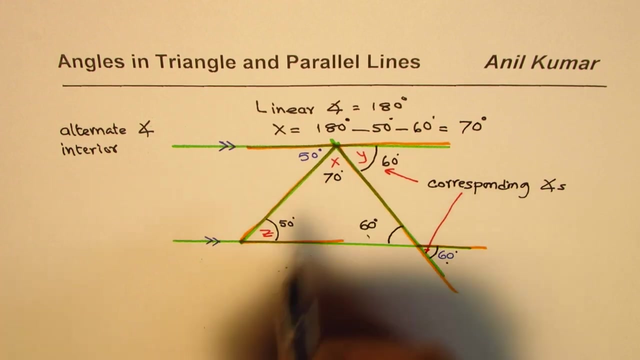 is equals to 180 degrees. the sum so x should be equal to 180 degrees. take away 50 and also take away 60 rights, so that is 110. you can use calculator to find the answer. you get 70 degrees. now here is a check. check for you. is that within a triangle, what is the sum of angles it should be? 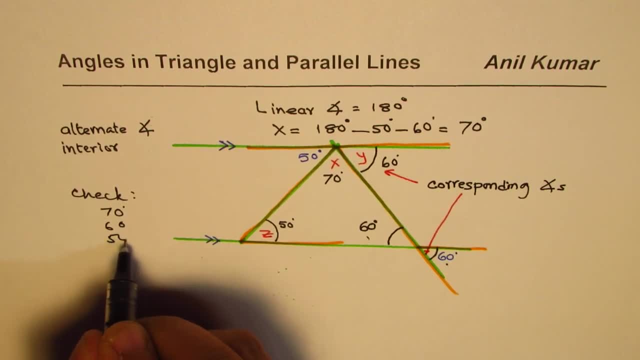 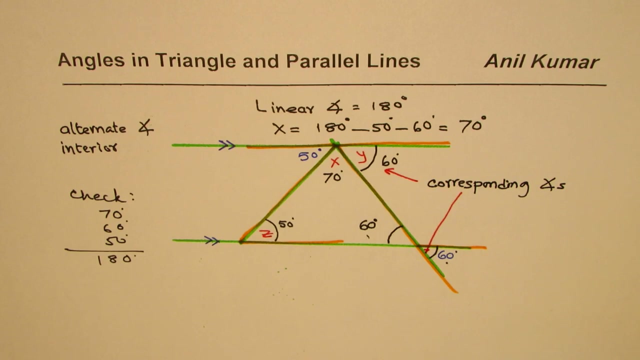 180. so you can add 70, 60 and 50 and check. you'll find this is 180 degrees. so that ensures that the calculations which you have done are perfectly fine, amandil kumar, and i hope that helps you to quickly get the correct angles. thank you. and the best.